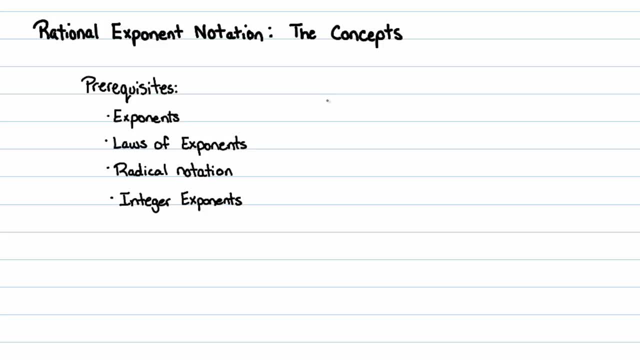 very familiar with radical notation- However- I'll talk about that a little bit here- And then extremely familiar with integer exponents, negative exponents and zero exponents. We'll first start this with just a review of what radical notation actually is. I debated 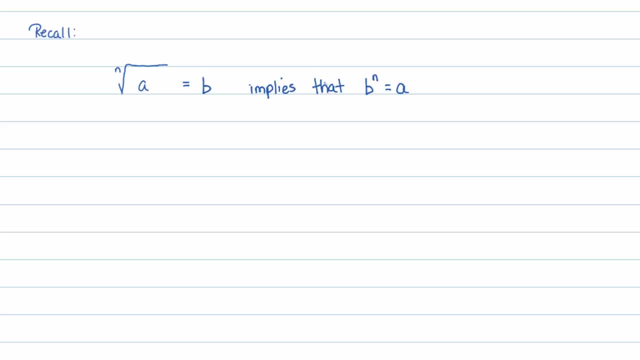 on how I was going to write this, and I decided with writing this as an equation. The nth root of a is equal to b. implies that b to the nth is equal to a. Now let me give you an example of what I mean, and then I'll talk about the parts of this. A simple example. 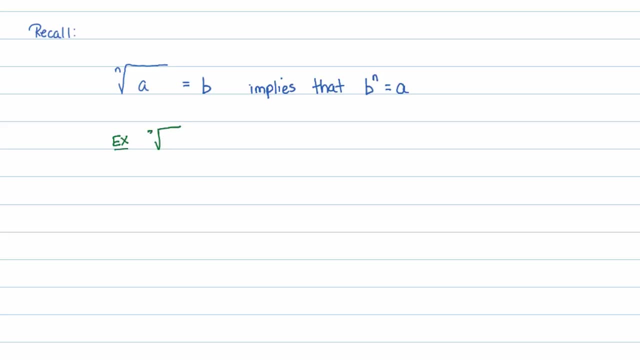 is that the third root of 27,. well, that happens to equal three. Why? Well, because I should do this? I'll say because because this three to the third power is equal to 27.. In other words, this three raised to that third power is equal to 27.. And in fact we could see: 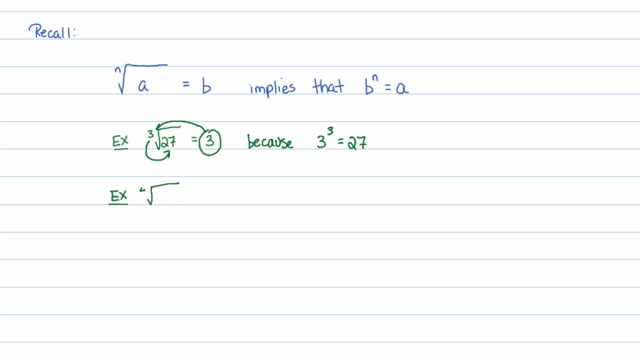 this in a lot of cases, like- let's do- the fourth root of 16.. That's equal to two. And the reason why is because two raised to the fourth power is equal to 16.. Again, two. and let me go ahead and circle this up: two raised to that fourth power is equal to 16.. So, raised, 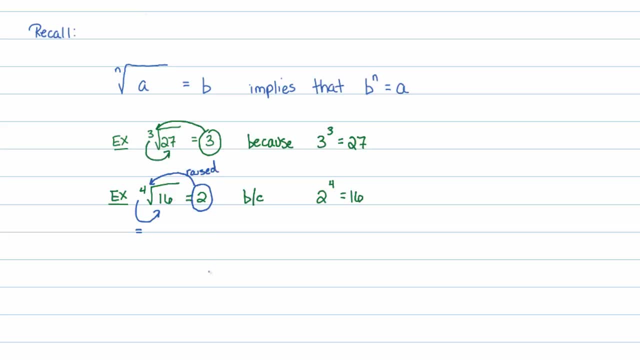 to two. raised to the fourth, power is equal to 16.. Now I want to. the reason why I'm kind of using this circular notation here is because I'm going to use this when we introduce a concept called logarithms in the 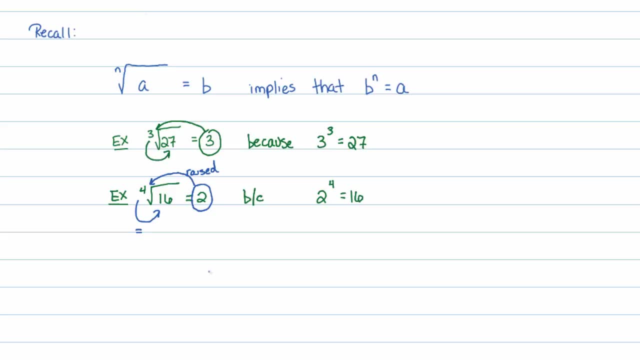 future. So I just want us to get used to this circular argument that these two notations imply the same thing. They're two equivalent notations. So when somebody says, oh, the third root of 27 is equal to three, you could say, oh, you mean three to the third power. 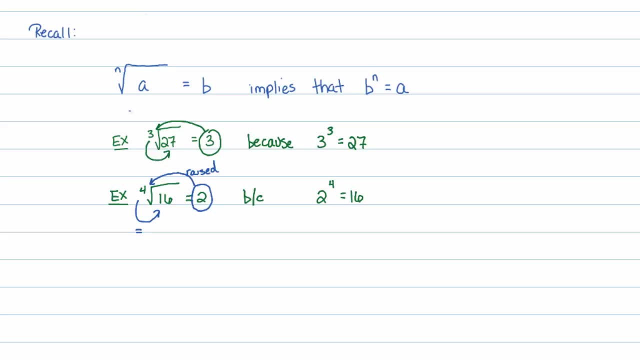 is equal to 27?. Or if somebody says, oh, the fourth root of 16 is equal to two, you could say, oh, you mean that two to the fourth power is equal to 16.. And in fact that's. 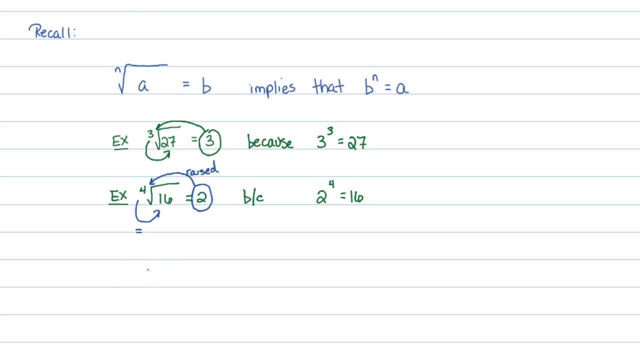 not true. In fact, we're often used to seeing negative or- I'm sorry, positive numbers underneath radical signs, but it doesn't have to be that way. You could say the third root of: oh, let's go. a negative eight That's equal to negative two. The reason: why is that negative? 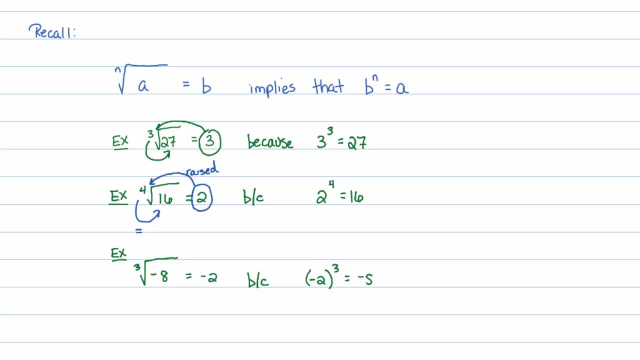 two raised to the third power is equal to a negative eight. Just look at that circular argument here. Negative two raised to that third power is equal to six. So that's a negative eight. That's equal to negative eight. I'll write the little raised two here I didn't write. 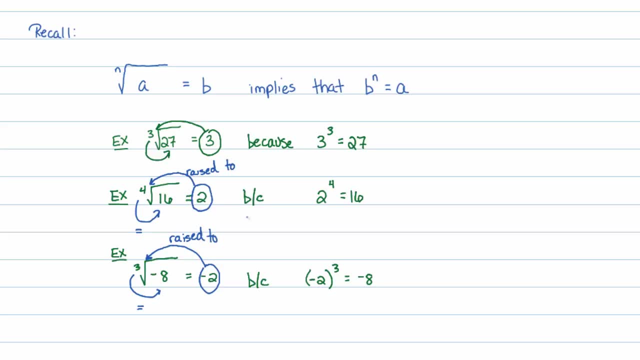 two right there but I should have. So that's a little review of radical notation that you should be very familiar with at this point. anyway, A couple definitions here. The n is called the index of the radical, And often we don't like indices of radicals to be anything. 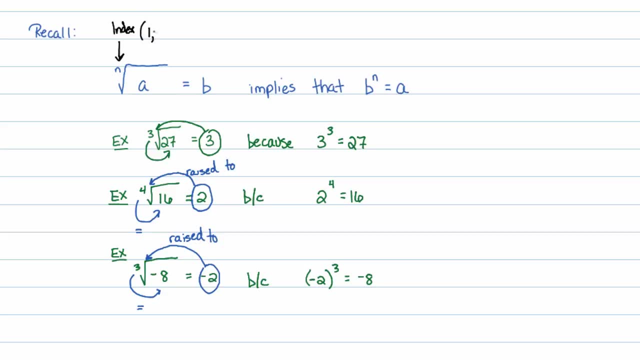 except for natural numbers. So this is numbers like one, two, three, four, five, six, seven, one, two and so on and so forth. The symbol itself is called the radical symbol, And the interior of that radical function, because that really is a function. I'm plugging something. 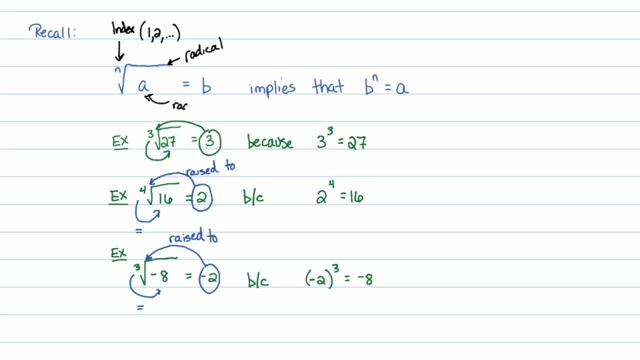 in. I'm getting something out is called the radicand. Now those are all definitions. I personally don't really care to know all the definitions, just as long as you know how to use them and can talk about them. So I decided to write down a few extra examples here because I think it's very important to 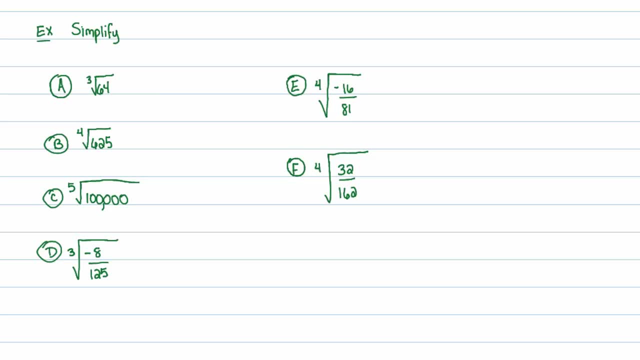 get some practice. So, each of these, we're going to go ahead and simplify And, again, following that idea of how to find the root of a number, here we'll go ahead. I often do this, So I'm going to go ahead and do this. So I'm going to go ahead and do this. 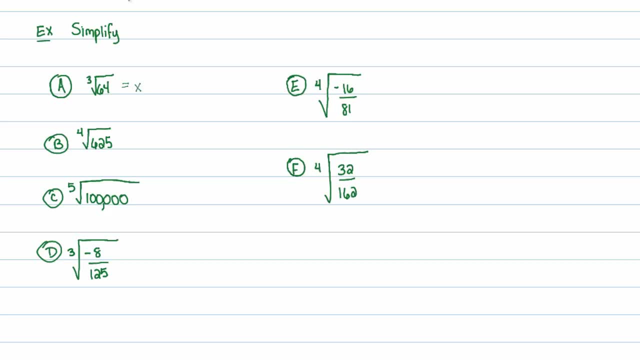 The cube root of 64 is equal to some number I don't know, And then I'll use that circular argument that x raised to that third power should equal to 64. So this is the raised to. I know it's maybe a little bit small unless you increase the size of this video. So this: 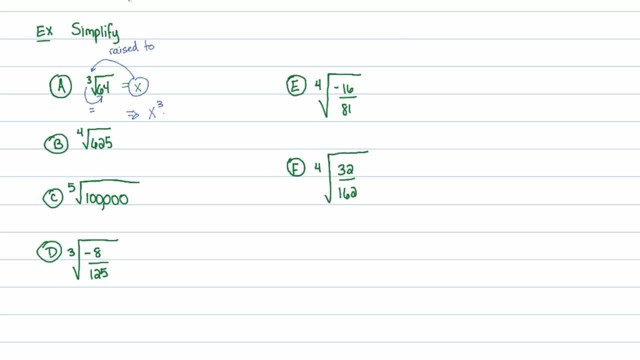 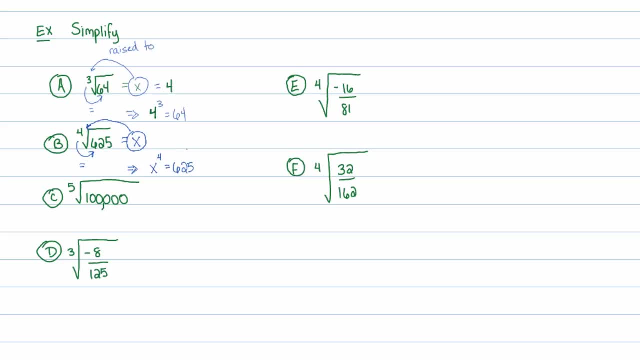 to 64. And we know that x raised to the fourth power should equal to 64. And we already know that 5 raised to the fourth power should equal to 65. That's exactly very difficult when you install the formula. But we know that 5 raised to the fourth power. 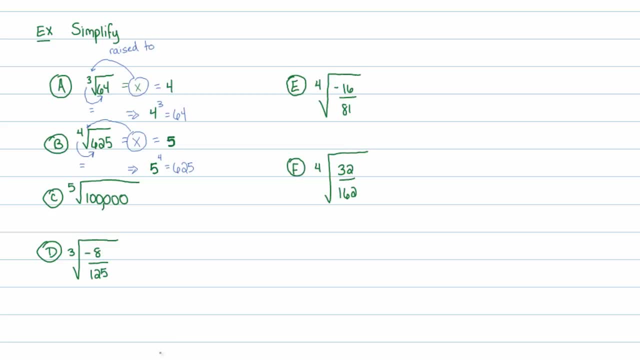 is equal to 65. And, based on this formula, we know that 9, raised to the fourth power is equal to 65. And we know that yours, producing the number 85, isn't worth 65. So if I want to calculate t, I'm going to use t equals 5.. Like, that's how you're going to do this. 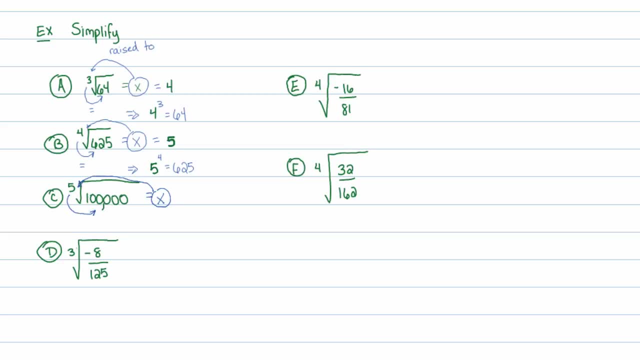 here it will equal 100,000. now, the clue to what this number is going to be is the fact that the that we're looking to raise a number to the fifth power to become a hundred thousand, and that's a power of 10, right there. 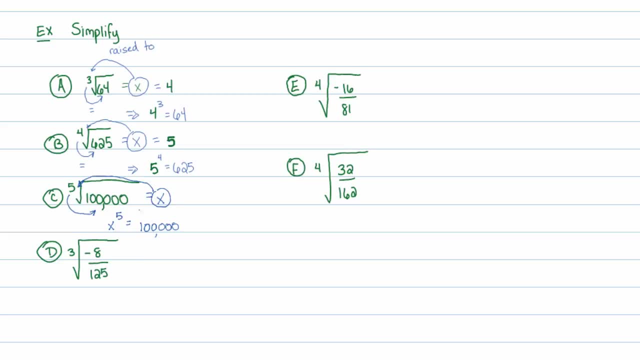 in fact, I'm going to guess that it's going to be 10. I'm thinking that the fifth root of a hundred thousand is going to be 10. let's check it out: 10 to the fifth power is one with five zeros after it and one with five zeros after it. 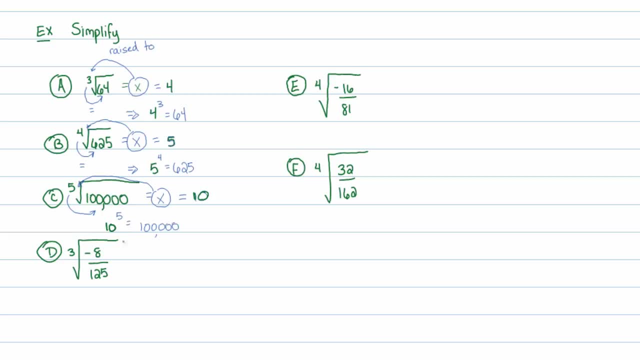 is one zero, zero, zero, zero, zero, which is a hundred thousand. so that does work out. and now we move on to this next example, this next example when I see something with a little bit of math inside of it. so here's a function. again, radicals are functions. 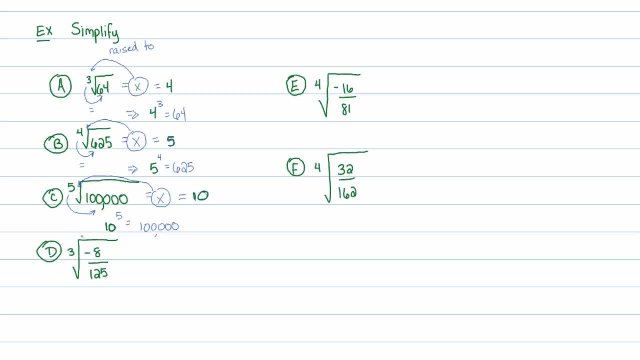 but this function has a fraction inside of it, a function with a fraction, and the first thing I want to do is simplify that fraction, if it can be simplified. so I'll see if there's any common factors between the numerator and the denominator, which there are not. so it's just a little check I do. 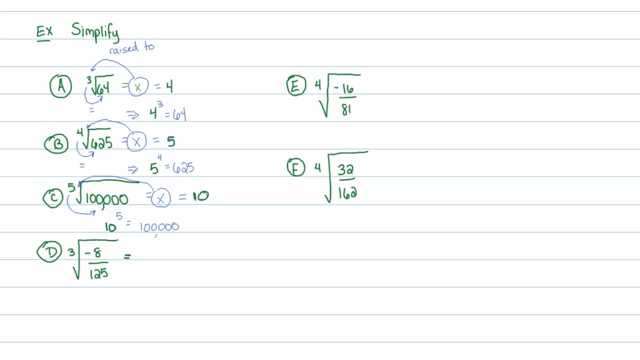 and then I ask myself: well, I know this is going to equal something, I just don't know what that something is. so I'll call that X and I'll ask myself: what do I raise to the third power to become a negative 8 over 125? 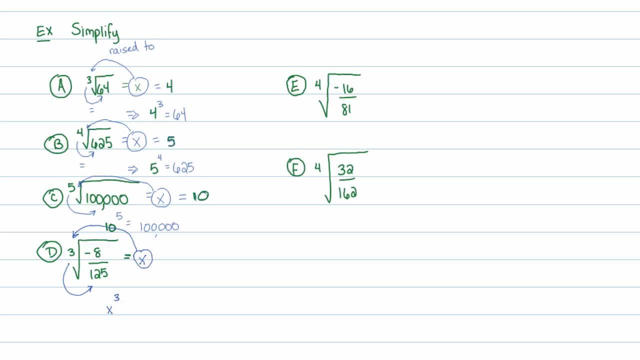 so what do I raise to the third power to become a negative 8 over a 125? first thing I'm going to notice here is that any number that I raise to a power, if I want that answer to be negative, that number inside that X should be negative. 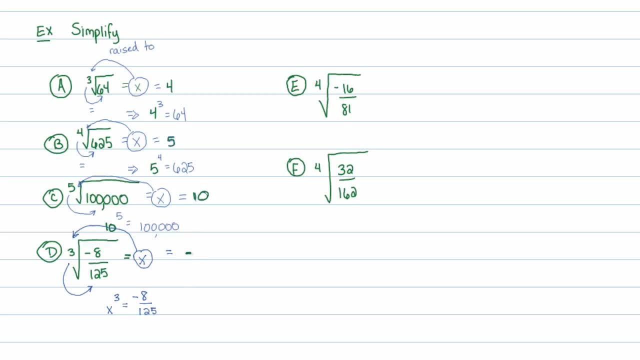 so I'm going to write a little negative sign out front and I'm going to double check that if X were negative, I'd have negative times, negative times, negative, which would definitely give me that negative right there. so we're okay, and now I need the numerator to become. 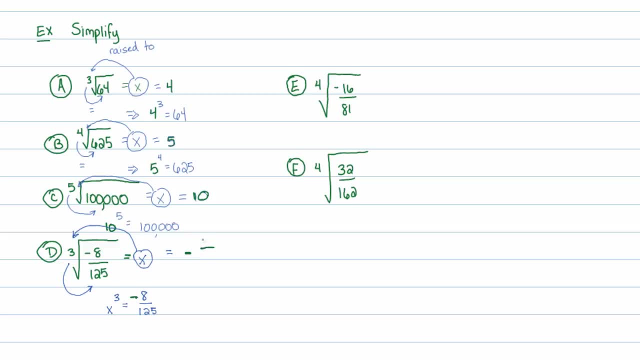 8. what number do I raise to the third power to become 8? well, that would be 2, and I need the denominator to become 125. what number do I raise to the third power to become 125? that would be 5. so therefore it must be true. 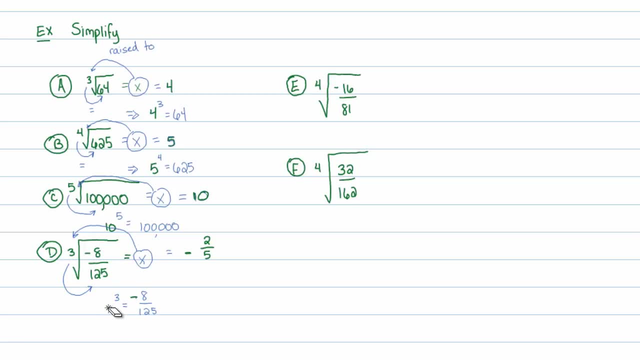 that the cubed root of a negative 8 over 125 is equal to a negative two-fifths. the reason why? because a negative two-fifths raised to the third power is equal to a negative 8 over 125. so I'm just using that circular argument the entire time. 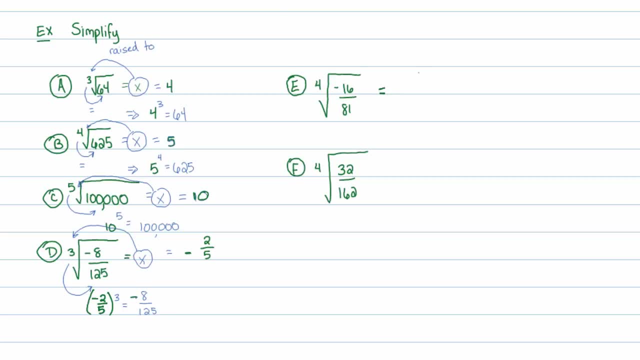 this next example, example E: here again I have no idea what it is, so I'll write X in here and I'll say: what do I raise what? what number do I raise to the fourth power to equal a negative? 16 over 81. so what number do I raise to the fourth power to equal a negative? 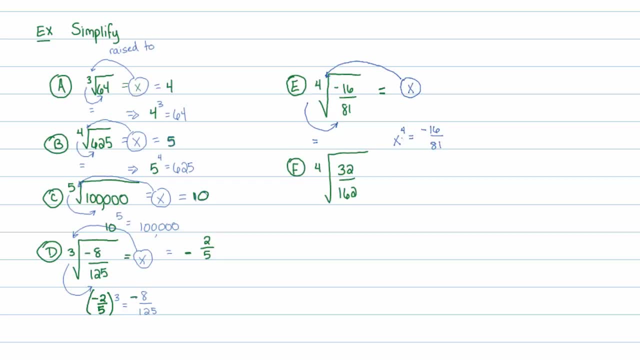 16 over 81 and you might notice immediately that there's no such number. because when you start taking even powers of numbers, if your number would have started as a negative number in here if X were negative, well, when you square it it becomes positive, when you cube it it becomes negative again, and when you raise to the fourth power, 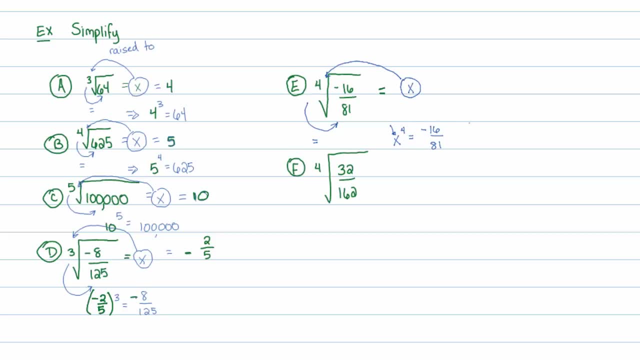 it has to become positive again. so there's no possible number, no such number, no way that we can get a number such that when I raise to the fourth power it becomes negative. so this answer there's. some people say no such number, that some people say it. 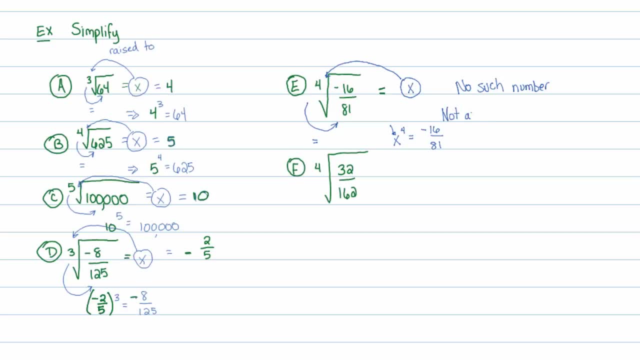 doesn't exist. it's actually not a real number. technically there is a number that that makes us true, but it's just not a real number. and for right now, let's just deal with real number. and for right now, let's just deal with real number. something I didn't say in that last example, but I will say it now in this: 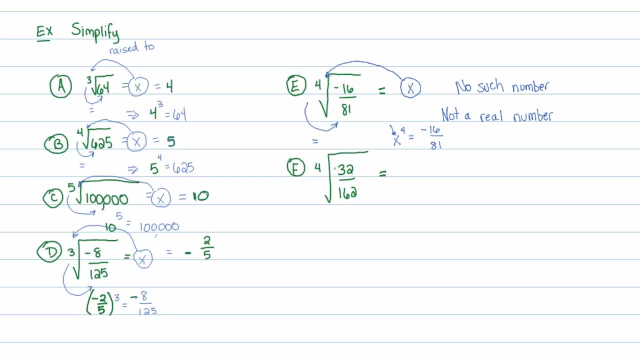 example f. this final example here is that, again, when I have a function in the inside, the function has a little math going on. I'll likely want to simplify it if I can. it might make my life a little bit easier. so in this case I see that I have a fraction. 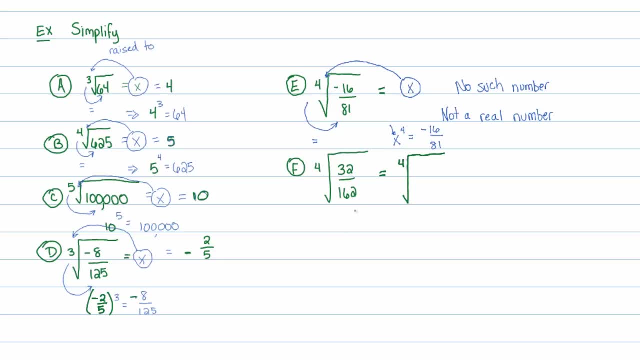 that actually will simplify because both numerator and denominator are divisible by 2. so in this case I see that I have a fraction that actually will simplify because both numerator and denominator are divisible by 2. If I divide 2 out of both numerator and denominator, I'll get 16 over 81.. 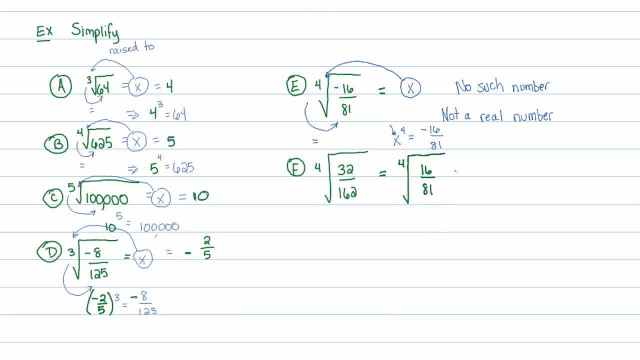 And now I know that that won't simplify any further. so I want to just find a value of x such that when I raise x to the 4th power, I will get 16- 81st. So let's see what that is. 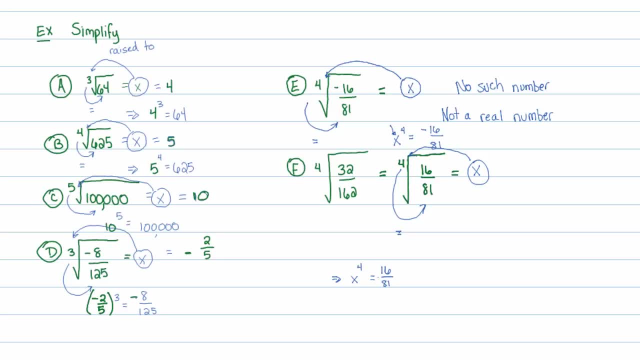 x to the 4th power. I want that to turn into 16- 81st And notice that this is almost the same question as before, but this time I'm actually asking when is x to the 4th power equal to a positive 16 over 81?? 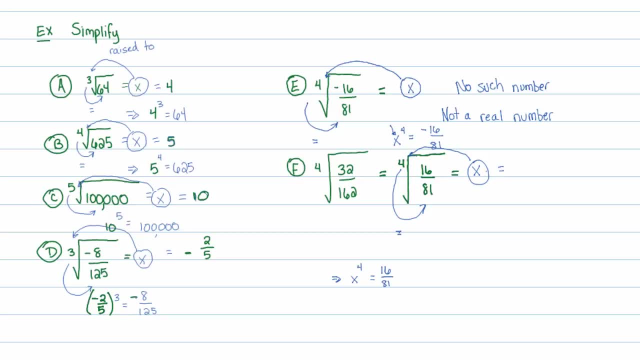 Well, I happen to know that for the numerator, a number to the 4th power that becomes 16 is 2.. 2 to the 4th power will be 16. And actually I should draw that in green here. And a number to the 4th power that equals 81 is actually 3.. 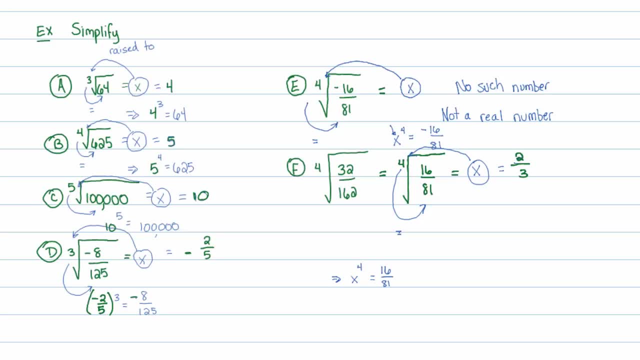 Turns out, the 4th root of 3,, 32 over 162, is 2 thirds. And again, the reason why is because, well, 2 thirds to the 4th power is equal to 16 over 81.. 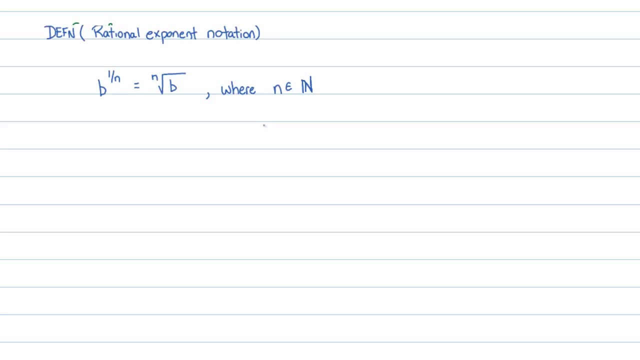 So, to get into the idea of what this section- or this lecture, I guess, is really focused on- is, since we're dealing with the concept of rational exponent notation. I'm not really going to do a lot of examples here, but I want to introduce the idea that 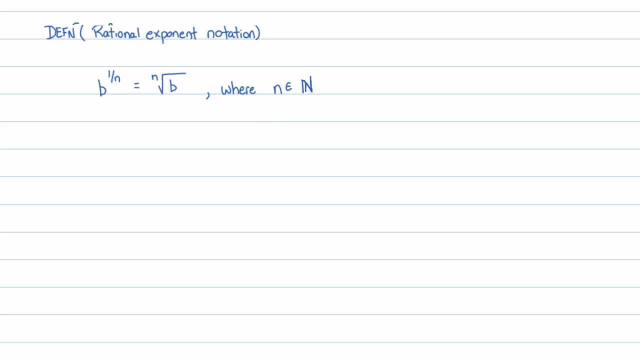 b to the 4th power is equal to 16 over 81.. So b to the 1 over n. so that's the exponent on that is 1 over n is defined to be the nth root of b, where n is a natural number. 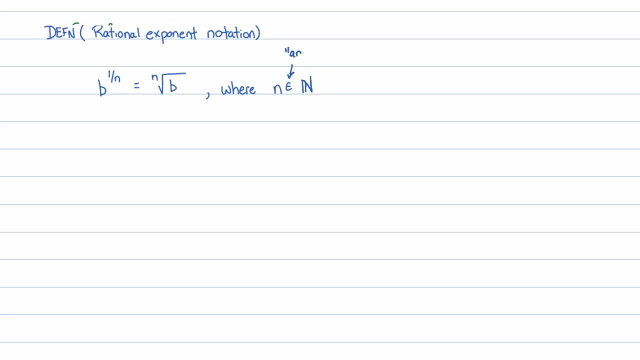 Now remember this notation here means an element of, and then that n with a bar on it is the set of natural numbers. So I'll write that in here. So, for example, 4 to the 1 half power is defined to be the 2nd root of 4.. 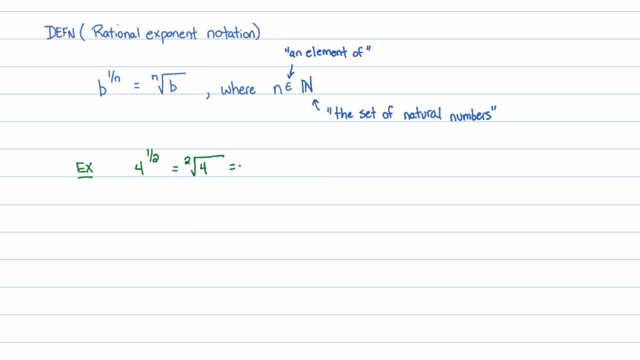 And we happen to know what that is. by the way, The square root of 4 is just 2.. Let's see 27 raised to the 1. third power is just defined to be the 3rd root of 27.. 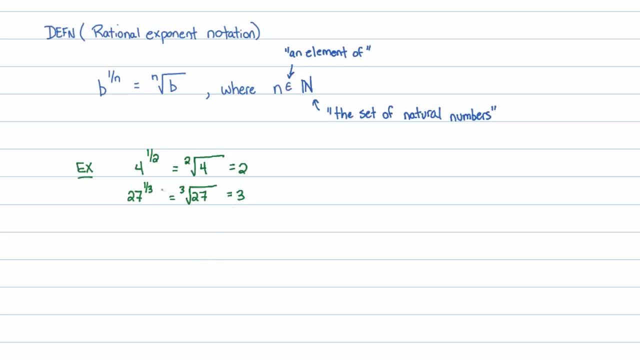 And we happen to know the 3rd root of 27 is 3.. And so on and so forth, And you could deal with larger powers and negative numbers. even So, negative 8 to the 1 third power is the 3rd root of a negative 8,. 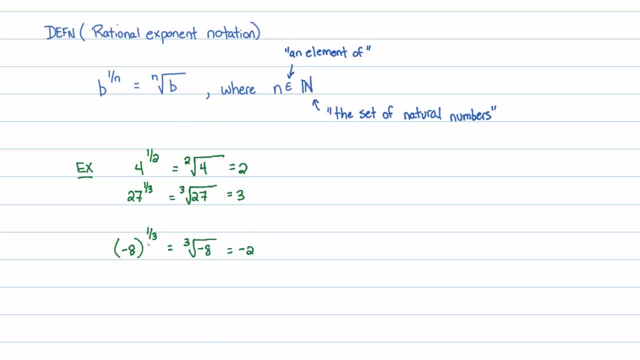 which will be a negative 2. Now this notation. a lot of people have a hard time and want to know why we've introduced this new notation. The new notation actually is a more powerful notation. Radical notation only works for a while in mathematics. 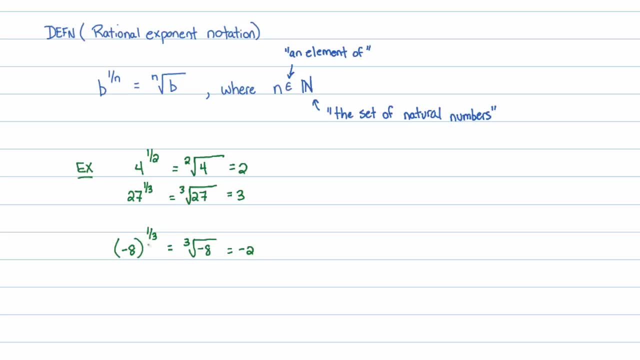 and then starts to fall apart. So I mean, it doesn't really fall apart. you could use it, It just gets bulky to use. So I highly recommend that you start thinking of rational exponent notation more than radical notation. So whenever you see somebody write something like: 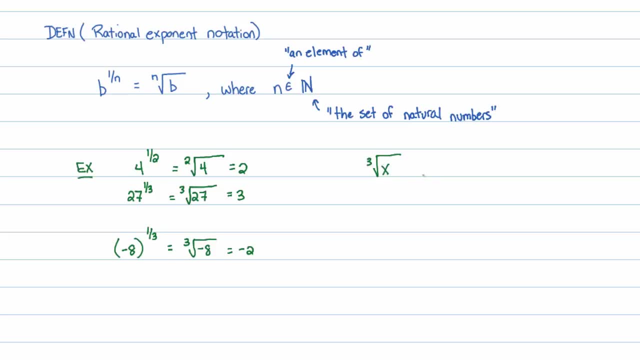 oh, I need to find the cubed root of some number, x. you could say: oh, you mean you need to find x to the 1 third. Yeah, that type of thing, It's just. it's very important because eventually you get to like the 7th root of some number. 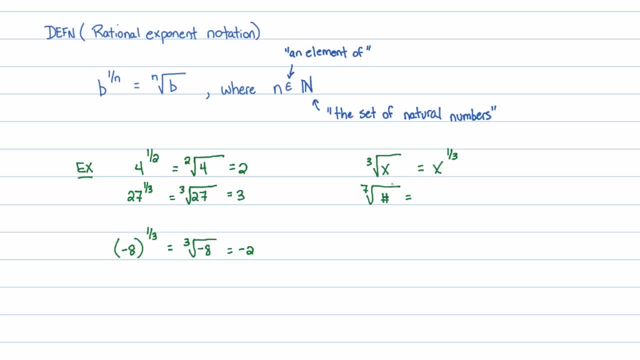 And that's just. it's so bulky to write. A lot of people don't understand what a 7th root is. A lot of citizens don't realize that you can even have a 7th root of a number, So it's much easier to say: 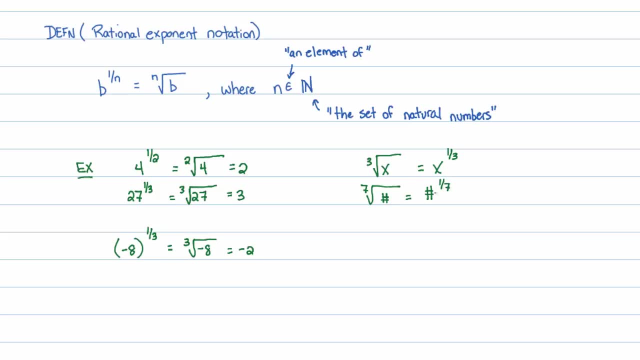 well, let's just write number raised to the 1- 7th power, Because that, for some reason, is a little bit easier to work with, to be very honest with you. So that's how rational exponent notation works, Now that I've kind of given you this idea. 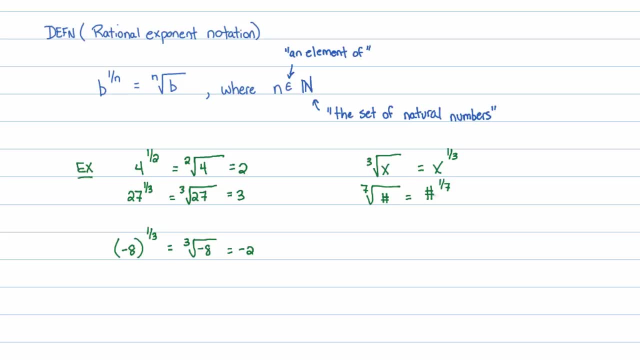 of what a rational exponent is and how the notation works. we're going to, in the next lecture, use it in examples, But before we do I want to introduce one, just one more little rational exponent notation definition. Not really a definition, more of a theorem. 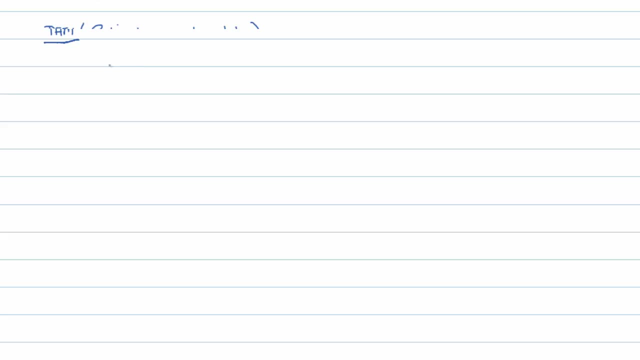 And I've decided to write this out as I talk about it. So every once in a while you get a radical. that's like the nth root of a number, let's say, And the number that you're taking the nth root of is a powered number. 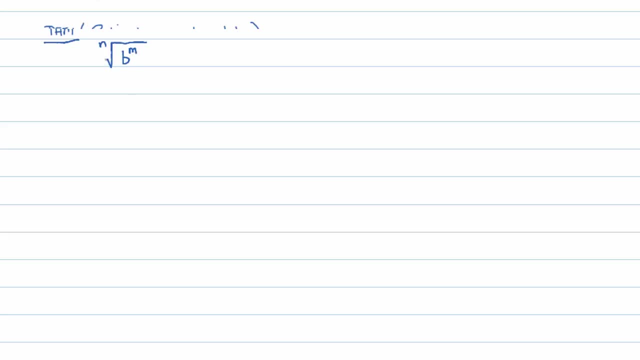 So, in other words, it's like b to the nth power. Well, we can write this using rational exponents and it's actually even. it looks better than this, to be honest with you. So let's see how that would look with rational exponents. 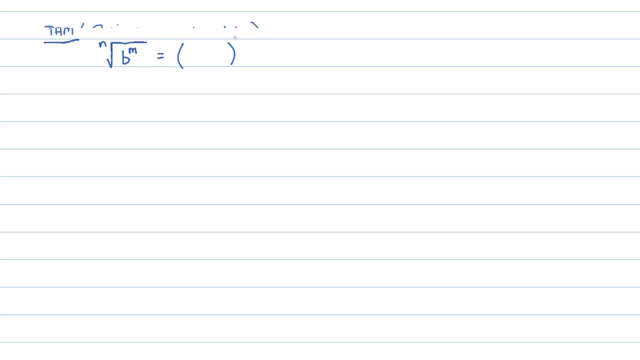 First of all, we know from the last slide, or the last page, that this is going to be b to the nth power raised to the 1 over n power. Right, Because the nth root just means the 1 over nth power. 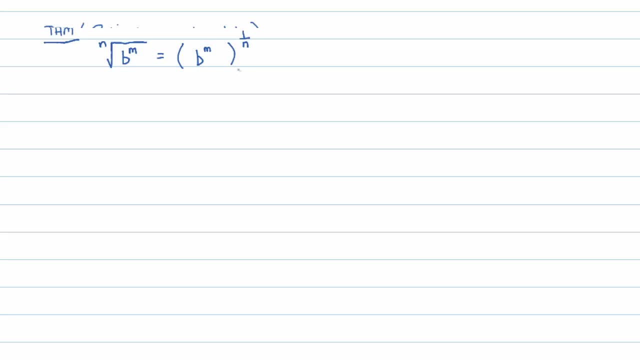 But now notice that this is b to the nth power raised to a power, And we know that we have that old theorem. let me write it over here- that b to the m raised to the p power is equal to b to the m times p. 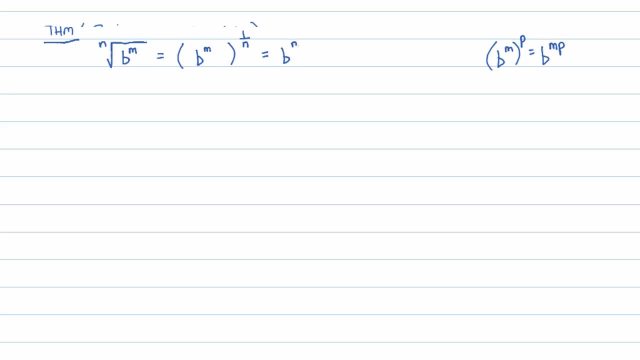 So this must be b to the m times 1 over n, or in other words b to the m over n. And what's great about this notation is that I see immediately in it that the n is the root that we were taking. 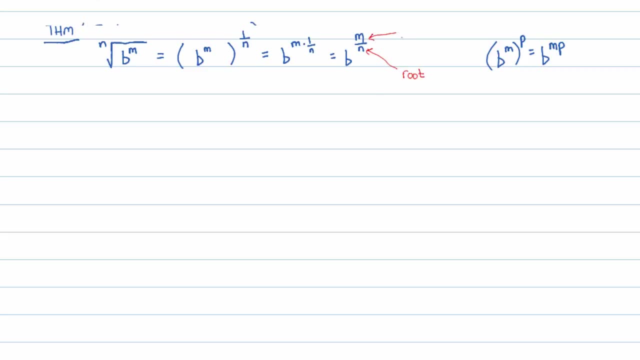 the nth root and the m, the numerator, is the power. So we were taking the nth root of b and raising that to the mth power. Well, technically we were taking b and raising it to the mth power and then taking the nth root of it.